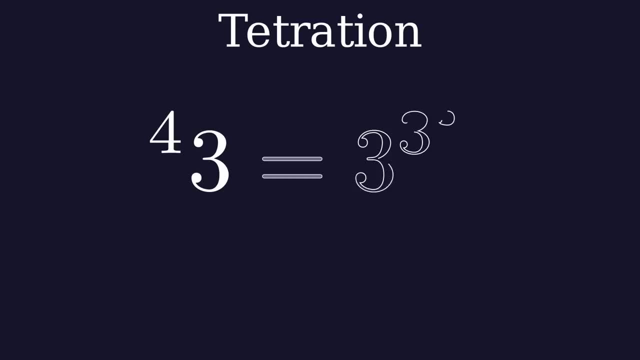 For example, 3 tetrated to 4 is a tower of 4 threes. To evaluate the tetration we always start from the top. So 3 to the power of 3 is 27.. 3 to the power of 27 is already equal to more than 7 trillion. 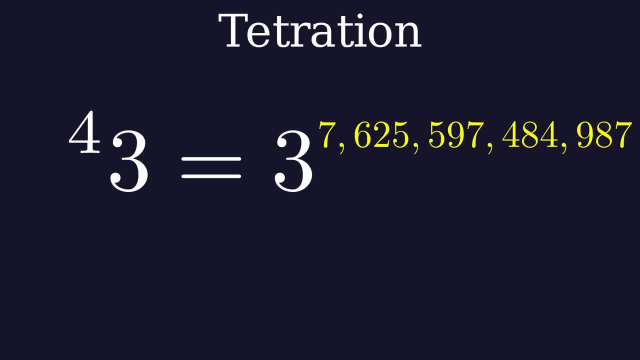 Multiplying 3 by itself, this many times results in a gigantic number. This number has over 3 trillion digits, With just the number 3 and 4, tetration can create numbers that are so enormous that it's hard for us even to imagine them. But tetration doesn't always have to generate numbers. 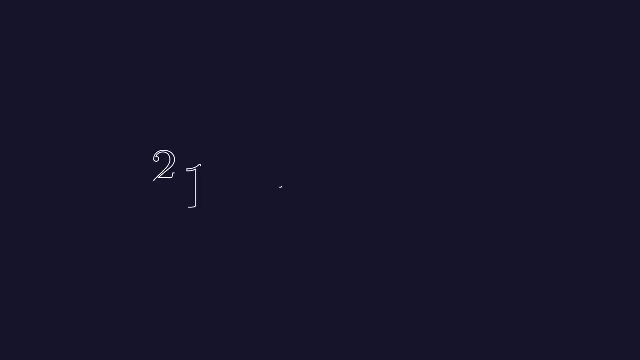 But tetration doesn't always have to generate numbers. But tetration doesn't always have to generate numbers. One tetrated to any number is always a one. One tetrated to any number is always a one. Even if we have an infinite tower of ones, it's still just one. 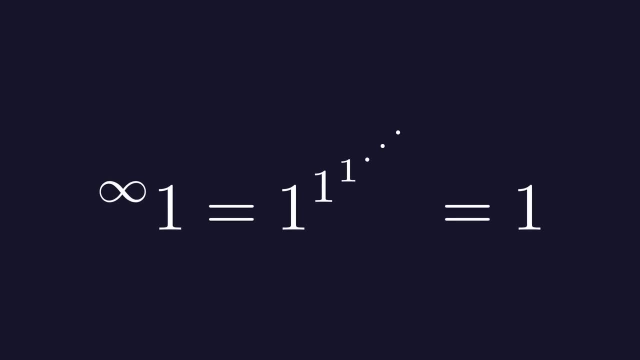 Even if we have an infinite tower of ones, it's still just one. This is a trivial example. but now consider an infinite tower of square roots of 2.. We can write it as the square root of 2, tetrated to infinity. 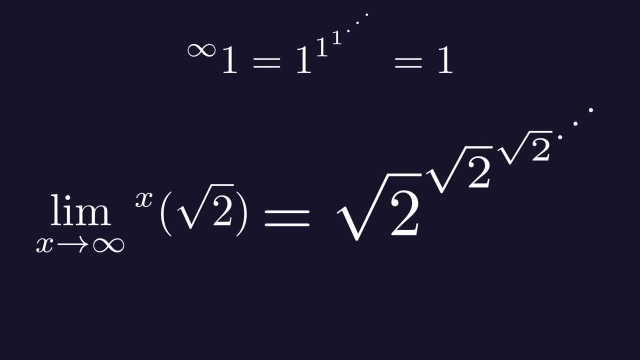 But a more accurate way to express it would be using a limit. as x approaches, infinity of the square root of 2, tetrated to x. Surprisingly, this infinite tower converges to 2.. The limit is x. precautions: infinity of the square root of 2, tetrated to x. 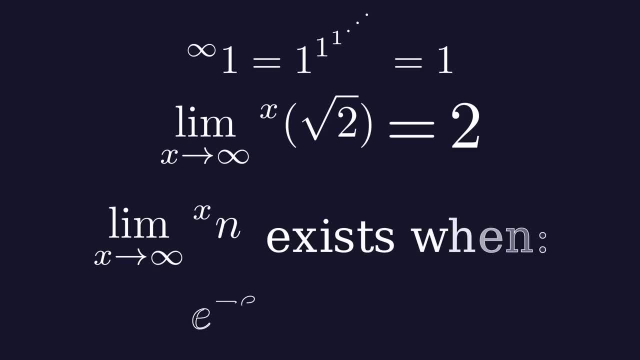 The limit exists when we tetrate a number that's between e to the power of minus e and e to the power of 1 over e, which is an interval from around 0.07 to 1.44.. The square root of 2 falls within this range. 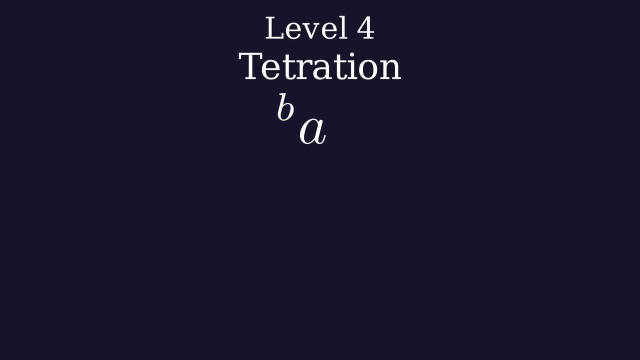 So far, we have written tetration using the left exponent. Unfortunately, there is no standard notation for tetration, but two up arrows are used very often and this notation will allow us to express even higher level operations beyond tetration. The arrow notation can be also used to write exponentiation. 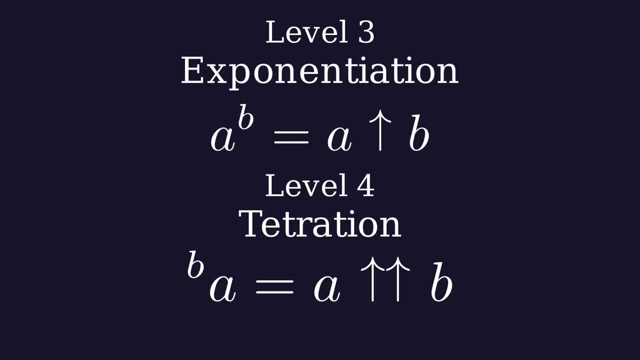 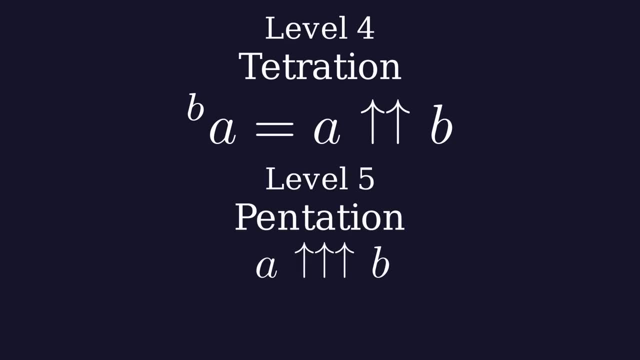 a to the power of b can be written as a up arrow b. With this notation, we can define an operation on level 5.. Using three arrows we denote pentation. Just like tetration is repeated exponentiation, pentation is repeated tetration. 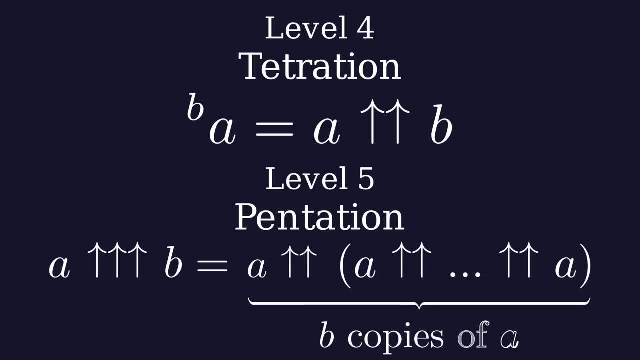 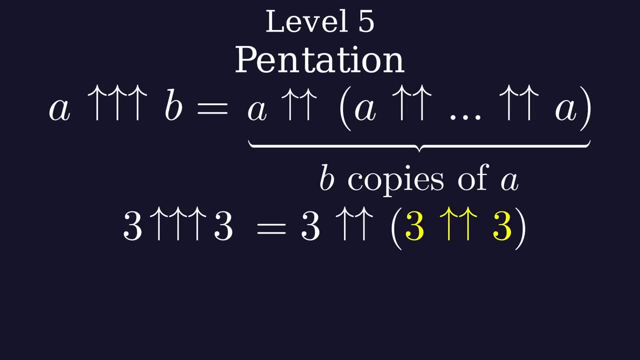 a pentated to b is equal to a tetrated to itself b times Three. pentated to three is equal to three tetrated to three tetrated to three and three tetrated to three is equal to three to the power of three to the power of three. 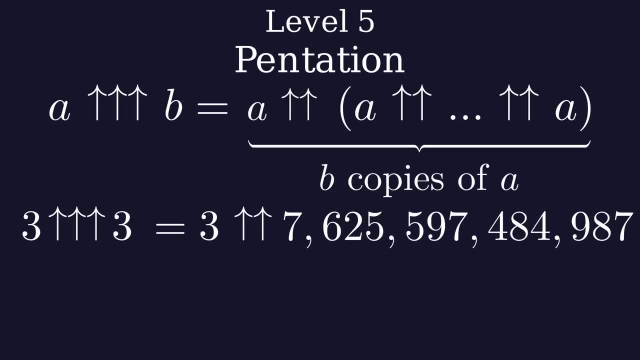 And that is equal to more than seven trillion And three tetrated to this number is a tower of threes of height- more than seven trillion. This number is unimaginably massive, But we can go a level higher. With four arrows we can denote hexation. 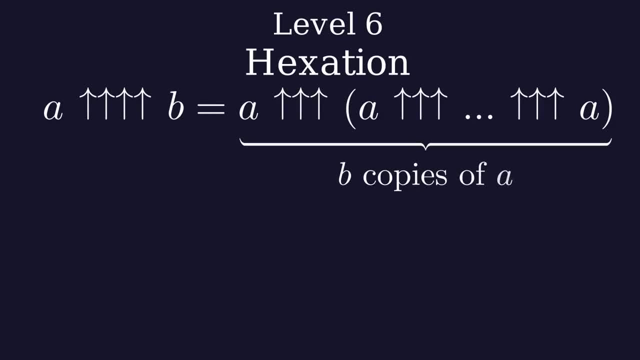 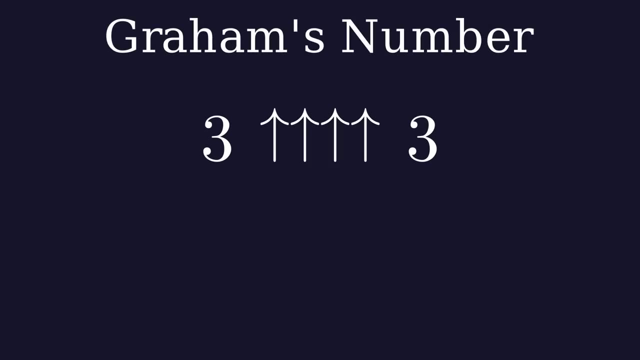 Hexation is repeated. pentation Three hexated to three is equal to three pentated to three. pentated to three. This number can't be compared to anything in the real world. With this giant number, we can start creating the Grohams number, which is one of the most 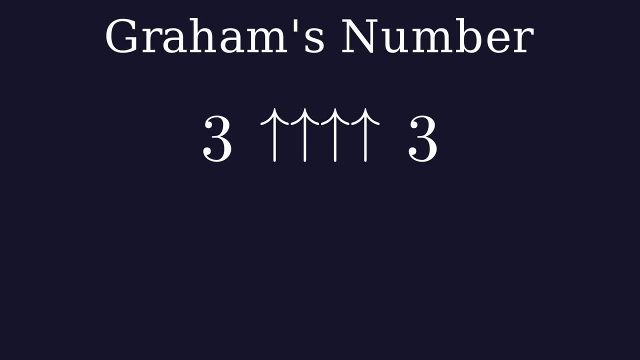 famous big numbers. To construct it, we start by defining that three hexated to three is equal to g0.. Hexation is denoted using only four arrows and already generates enormous numbers. But g1 is equal to three, followed by g0- number of arrows- and another three. 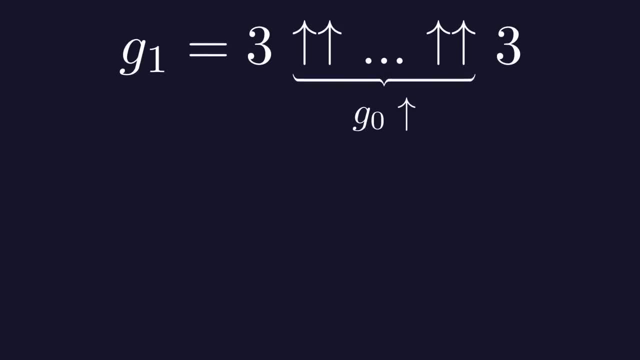 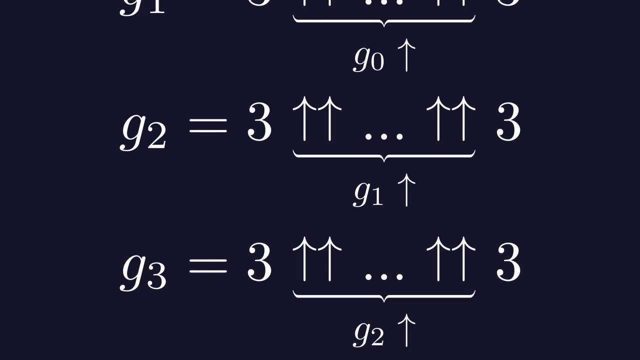 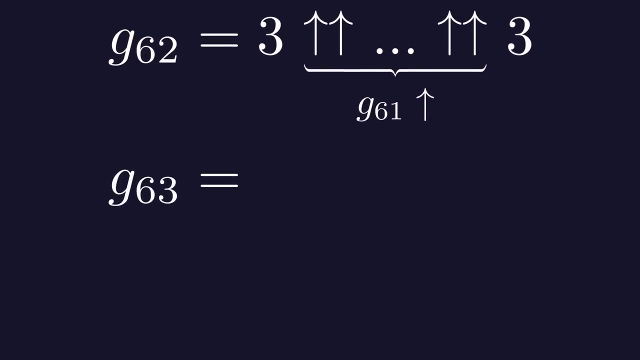 Just imagine how big this number is. Next we have g2, which is denoted using g1 number of arrows. g3 is equal to three. g2: number of arrows and three. This sequence continues until we get to the g63, which is equal to three, followed by g62. 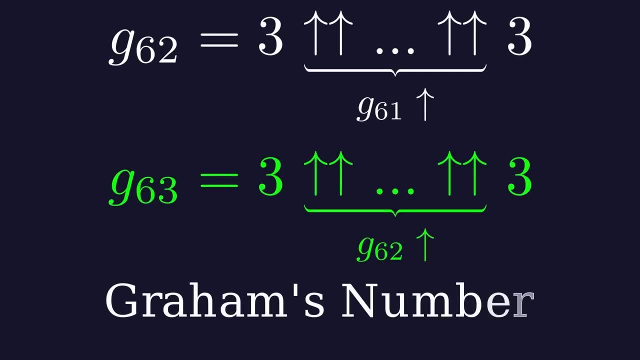 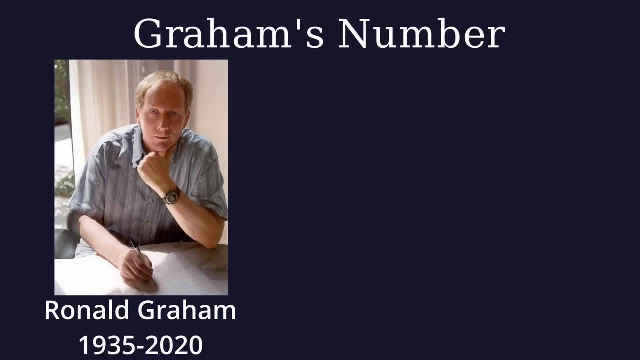 arrows and three. That is the Grohams number. Grohams number was used by Ronald Groham as a simplified explanation of the upper bounds of the problem he was working on. In the time of its introduction it was the largest specific positive integer ever to. 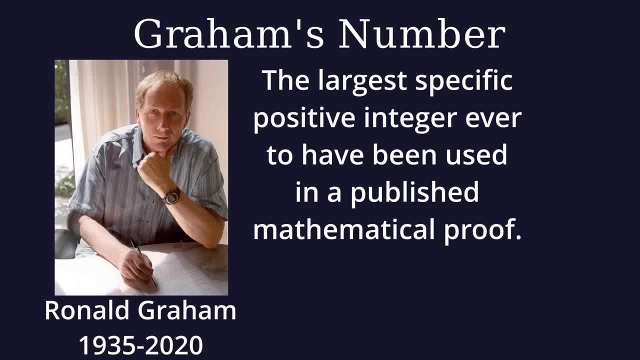 have been used in a published mathematical proof. In 1980, Grohams number was described in the Guinness Book of World Records. Since then, many bigger numbers have appeared in mathematical proofs. For example, the Grohams number is extremely small in comparison to the tree of three. 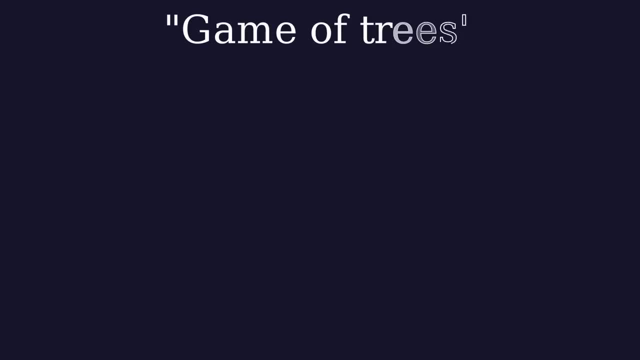 To explain what this number is, we need to play a game of trees. In this game, we try to create a forest using colored seeds following two rules. The nth tree can't have more than n seeds, The first tree can have only one seed, the next can have more than two, and so on. 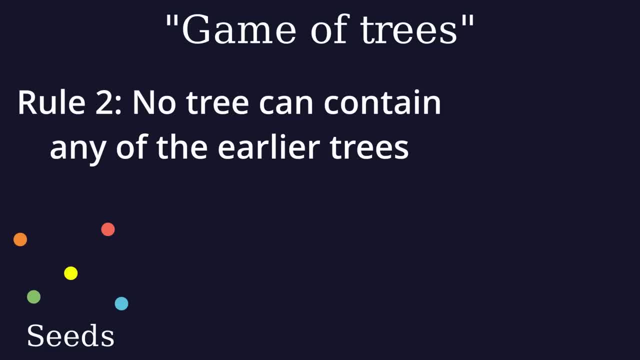 The second rule is that when you try to build a tree, it cannot contain any of the earlier trees within itself. For example, this tree contains this one, so it cannot be built. Also, the tree is contained in another tree. This tree is also contained in another tree. 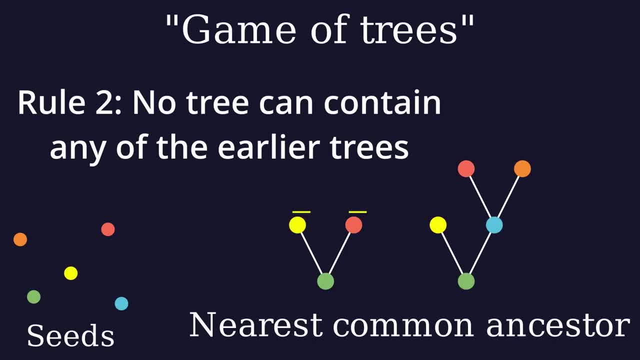 In this tree, the nearest common ancestor of the yellow and red seeds is the green seed. In the other tree, the nearest common ancestor of the yellow and red seeds is also the green seed. It means that the first tree is contained in the second tree, so the second tree cannot. 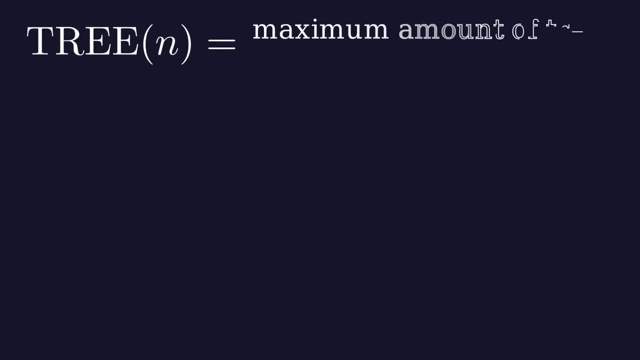 be built. The treeofn function tells us how many trees we can build using n colors of seeds. Using one color, we can only build one tree, Because the first tree will have one seed and any further trees would contain this tree. 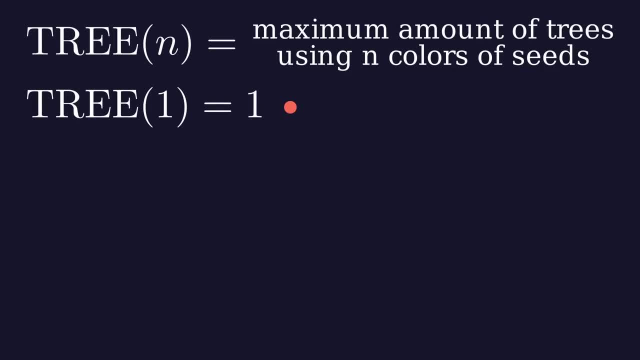 So treeof1 is equal to 1.. When we have two colors of seeds- red and green- the first tree has one red seed. the next can have any red seeds because it would contain the first tree. so we can use two green seeds. 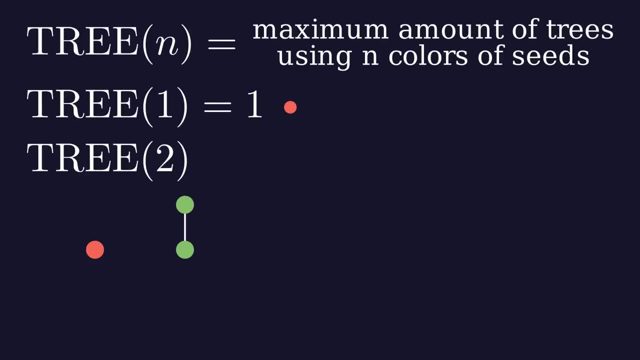 To build the next tree. we still can't use the red seeds. we also can't use more than two green seeds, But the third tree can have at most three seeds. so it can have only one seed and it can only be a green seed. 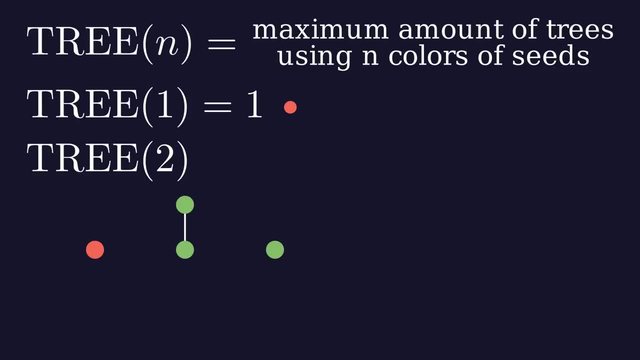 We can't build any more trees, so treeof2 is equal to 3.. Using three colors of seeds, we start with a tree that has only one seed. then we can have this tree, then another one, then another one, and all of them obey the rules of the. 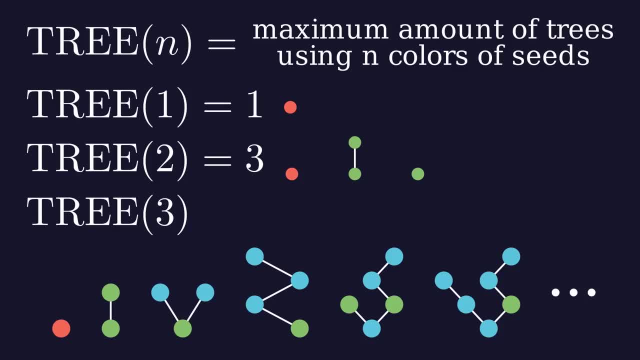 game, And we can go on and on and build more and more trees. The total number of trees we can build using three colors of seeds is equal to treeof3.. This number is very massive, even when compared to Graham's number, but we know that it is. 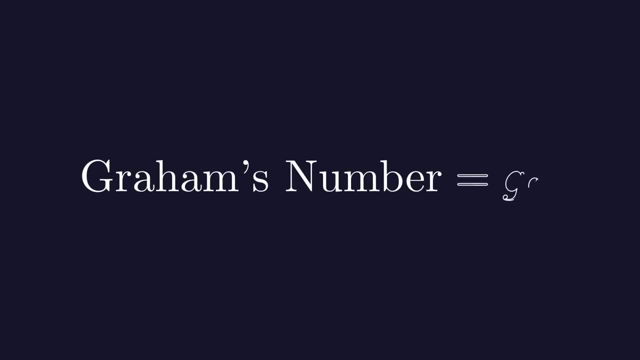 finite Graham's number, denoted as G63, is a colossal number, But we don't have to stop at G63.. We can keep going – G64 is defined as 3, followed by G63 arrows and another 3..